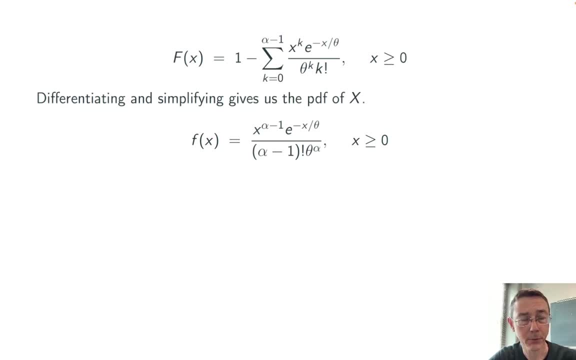 denominator. Since x is modeling waiting time, here the random variable x, the support is going to be only positive values, so x greater than or equal to zero. Now it's fine to have alpha be an integer and to use factorials when we're talking about waiting time, but sometimes the gamma 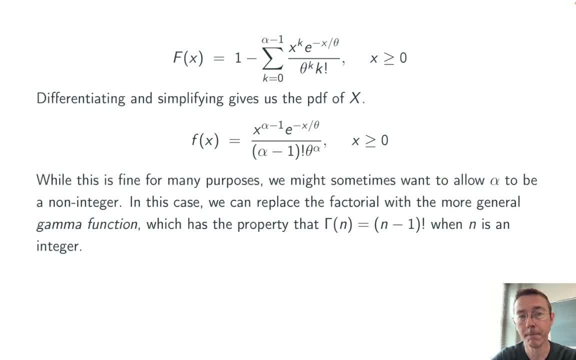 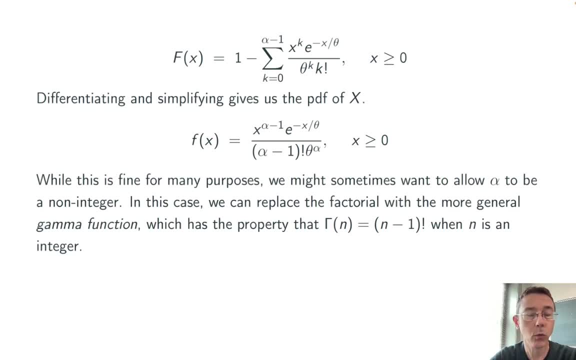 not have to require that alpha be a positive integer. So we can generalize this factorial function using the gamma function, And the gamma function is a mathematical construct that just agrees with the factorial on the positive integers. In fact, gamma of n is n minus one. 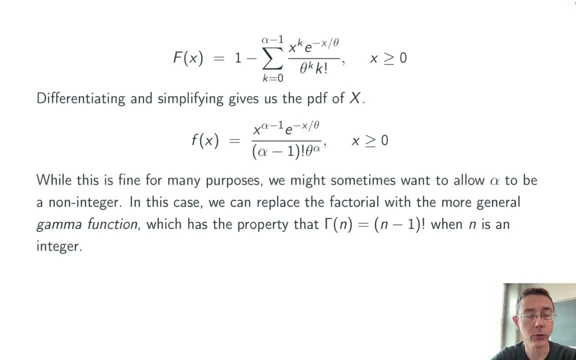 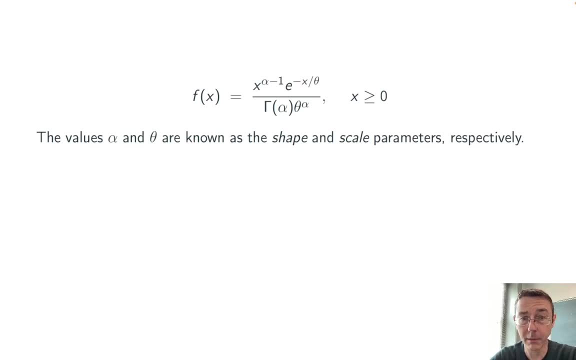 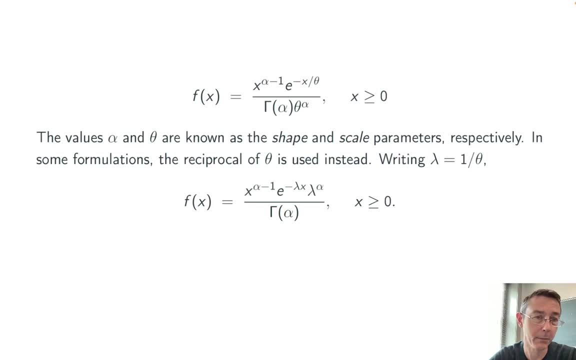 one over theta to get this formulation. It's somewhat less common, but you will see it. In particular, R uses this formulation when doing its calculations. Remember: theta is representing the average time between occurrences, And so it's reciprocal. lambda is going to represent the average number of occurrences per unit time. so that's that. 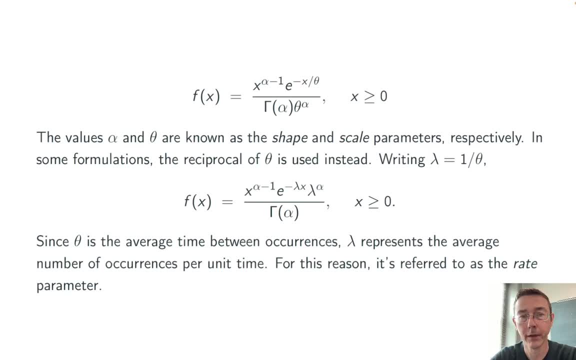 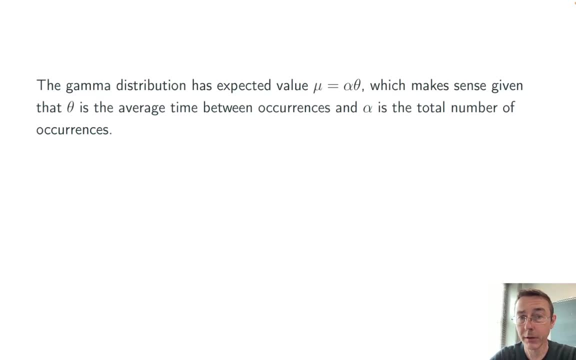 parameter is directly coming from the underlying Poisson process. because of that fact, lambda is often called the rate parameter. the gamma distribution has expected value. mu equals alpha times theta, and that makes sense, since theta is the average time between occurrences and alpha is the total number of occurrences. so the expected waiting time for alpha occurrences. 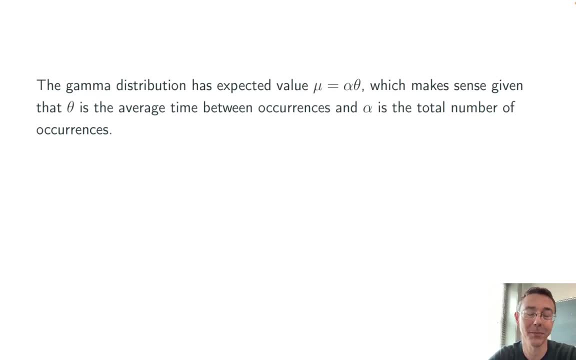 is just that number, alpha times the waiting time per occurrence makes sense. the variance formula is a little bit less memorable. it's alpha times theta squared. each of these can be proved using the moment generating function. m of t equals one over one minus theta. t quantity to the alpha. 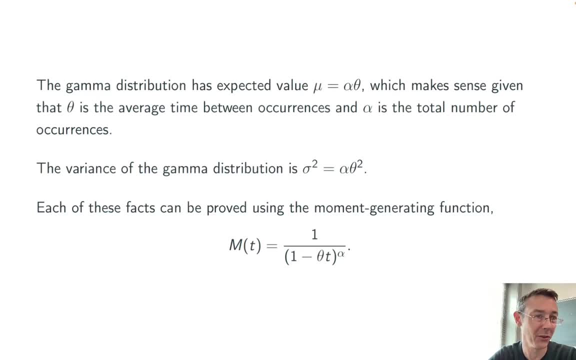 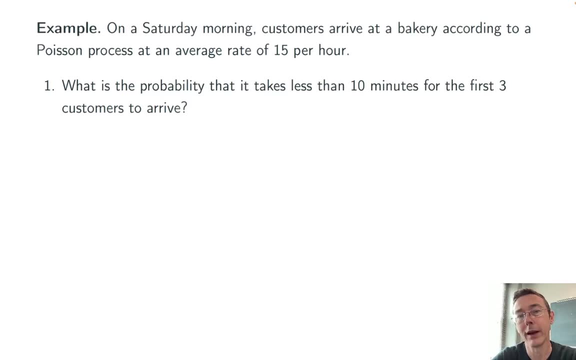 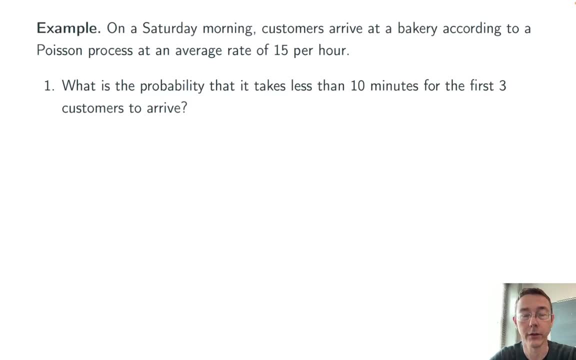 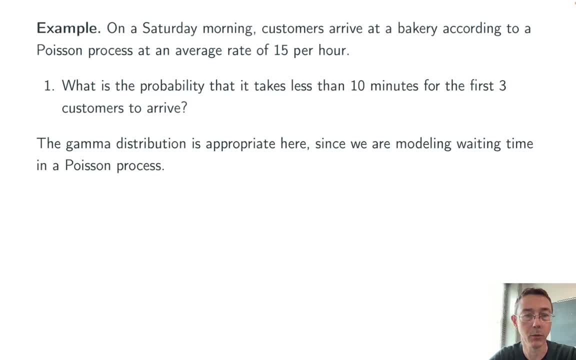 distribution is going to be appropriate here, since we're modeling waiting time in a Poisson process, since 15 customers arrive every 60 minutes, one arrives every four minutes on average. so that's our first parameter. theta is equal to 4 here, the average time between occurrences. the other parameter here: 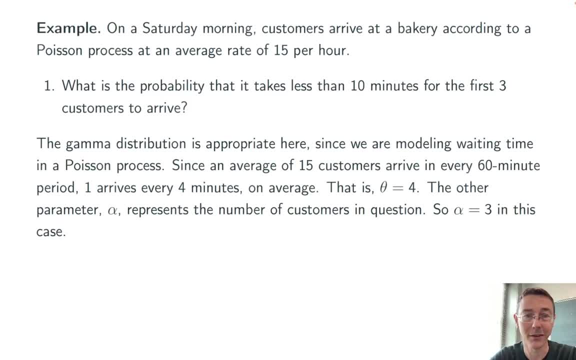 alpha is the total number of occurrences in question, the number that we're interested in. so here alpha is equal to 3.. okay, so now that we've got both of our parameters, we have our probability density function. we can get our total probability here by doing an integral. so the probability that 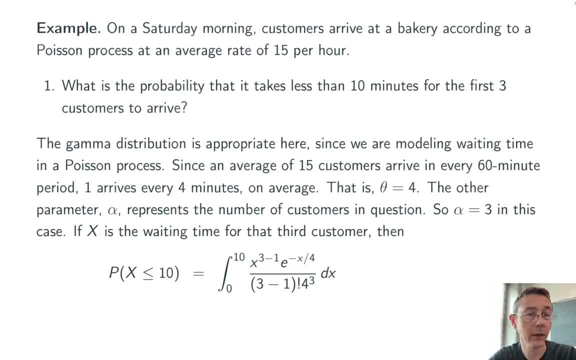 the total waiting time is less than or equal to ten. is the integral from zero to 10 of that pdf, and here i've just taken the pdf of the gamma function plugged in: alpha equals three, theta equals four. We can do this integral by integration by parts, if we have to. 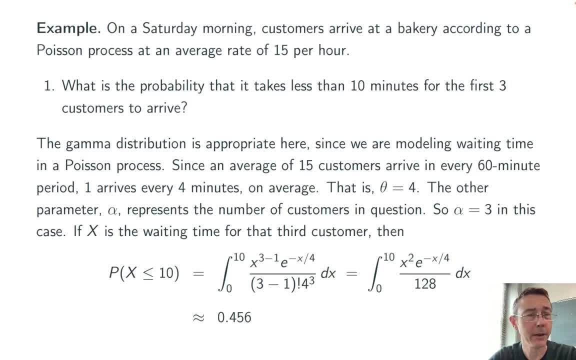 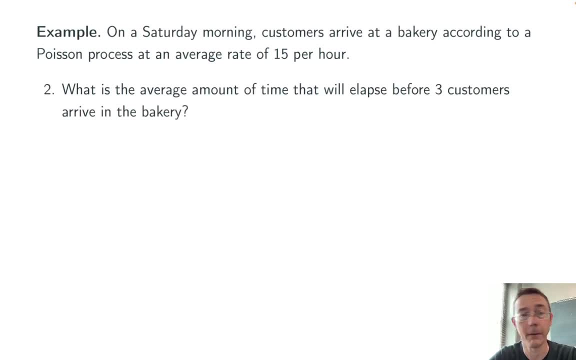 Using technology like a Wolfram Alpha is better. In my next video I'm going to show how to get this probability using r, using the p-gamma function. Once that video is ready, I'll throw a link to that up top as well. 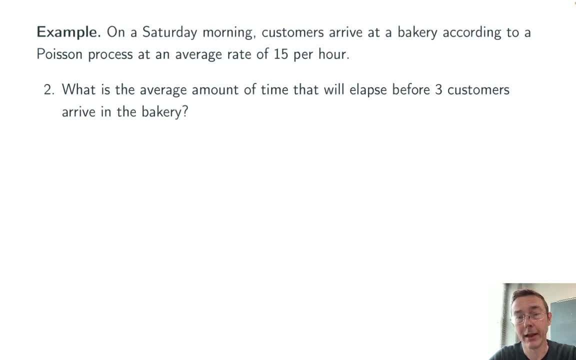 Problem two: What's the average amount of time that will elapse before three customers arrive at the bakery? So here we're just trying to get the expected value of that same gamma distribution. So we're going to use that formula from a few slides ago. 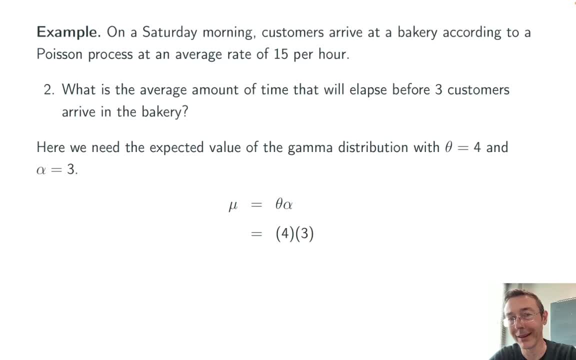 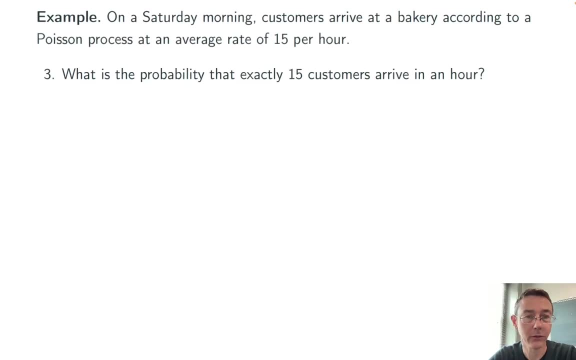 Mu is equal to theta times alpha, 4 times 3, about 12 minutes. Problem three: What's the probability that exactly 15 customers arrive in one hour? Now, in this case, we're talking about the number of customers that arrive in a fixed amount of time. 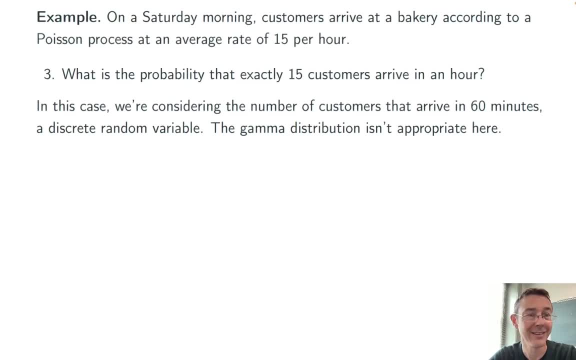 So the random variable here is actually the number of occurrences, not the waiting time. So the gamma distribution is not the best way to go about this problem. Instead we should use the Poisson distribution directly. So Again, I'll throw a link up top to that once again.